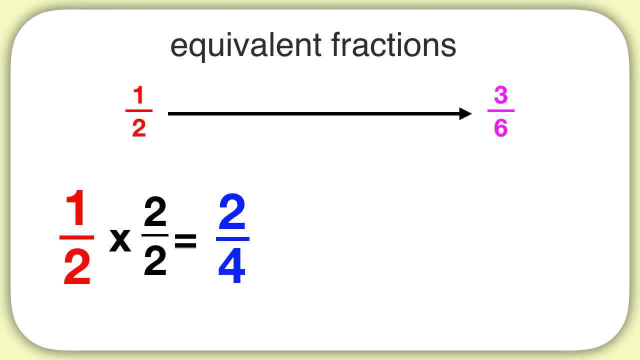 but what if I wanted to make 1 half 3 sixths? Well, we can take 1 half and let's multiply by 3 over 3.. 1 times 3 is 3, and 2 times 3, that's 6.. 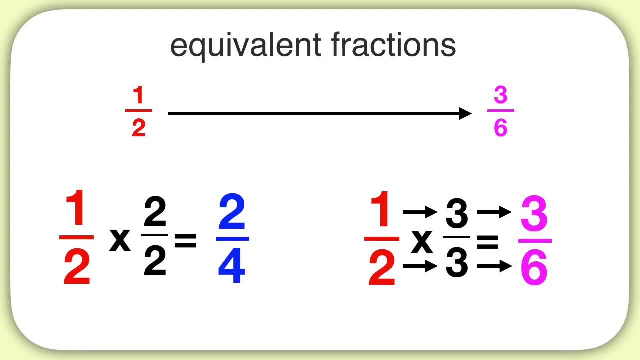 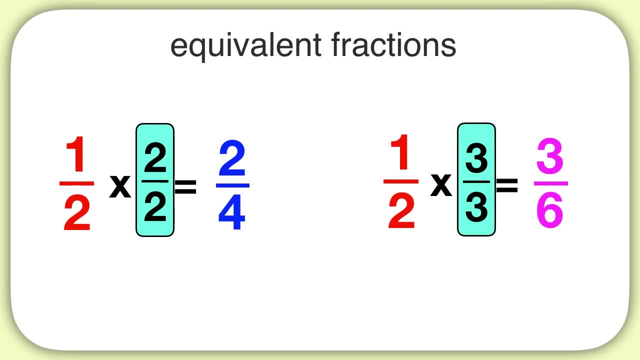 There you go. There is our equivalent fraction: 3 sixths. So now let's notice. To find equivalent fractions, we took 1: half and we multiplied both the numerator and the denominator by the same thing. To find an equivalent fraction, all you need to do is multiply the numerator and 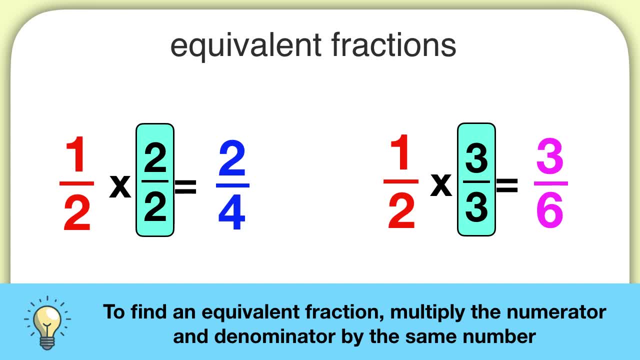 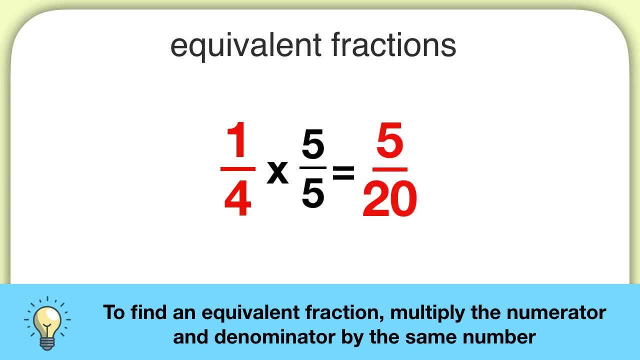 the denominator by the same number. For example, if we wanted to find an equivalent fraction of 1. fourth, all we would need to do is multiply the numerator and denominator by the same thing. We could pick any number like 5 over 5.. That would give us 5 twentieths, and because we 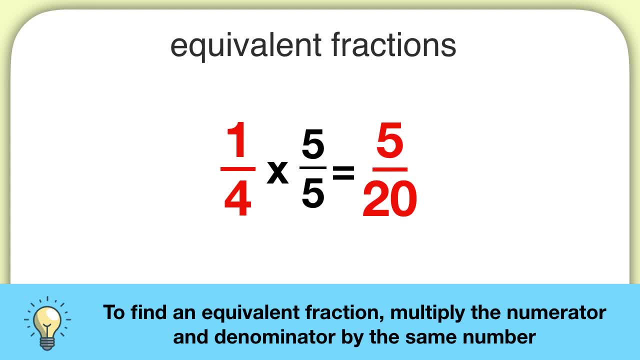 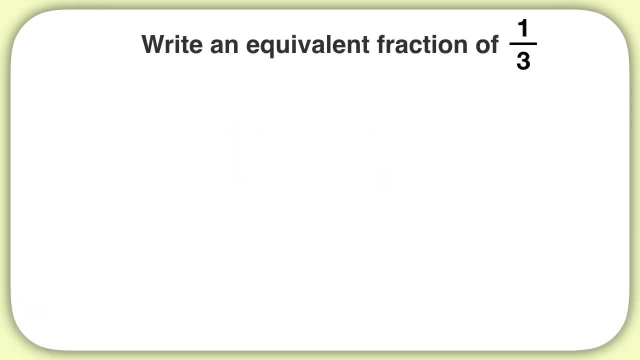 multiplied the numerator and the denominator by the same number, we know 5 twentieths will be equivalent. Let's practice one of these together. We're going to write an equivalent fraction of 1 third. Well, how can you make an equivalent fraction? We'll take our fraction. 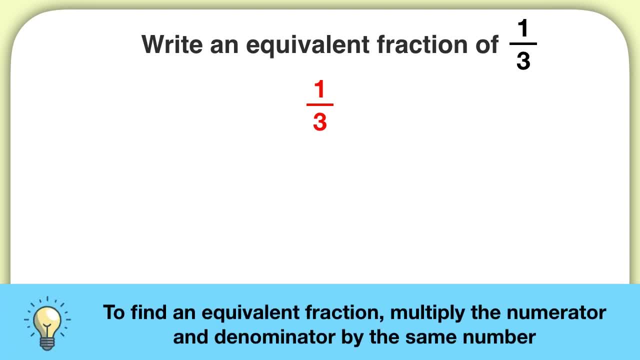 of 1- third, and then, to find an equivalent fraction, we multiply the numerator and denominator by the same number. We'll take 1- third and multiply it by something like 2 over 2.. What does this equal? Well, 1 times 2 is 2, and 3 times 2 is 6.. This is the equivalent fraction. 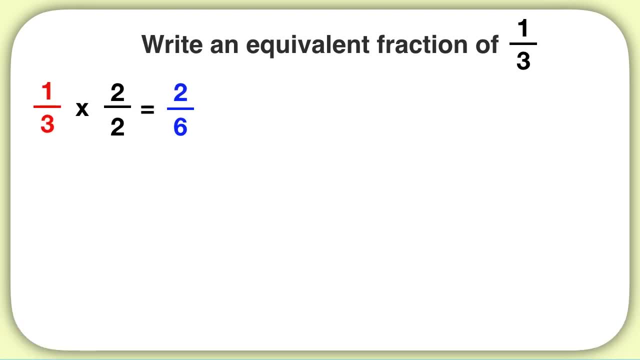 2 sixths. Let's do another. We could also take 1- third and multiply by 3 over 3.. What does this equal? Well, 1 times 3 is 3, and 3 times 3 is 9.. This is the equivalent fraction. 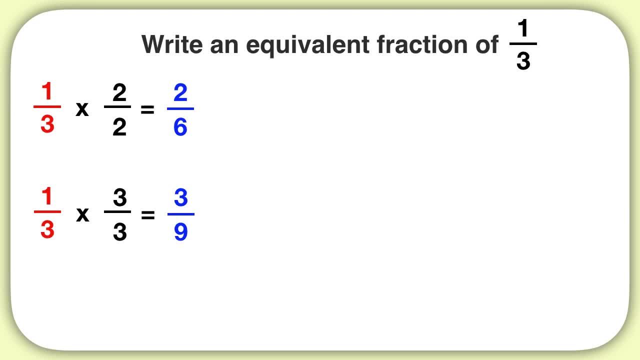 3 ninths. You can multiply by any number, as long as both the numerator and denominator are multiplied by the same thing You could do 1 third times 5 over 5.. That would give you: 1 times 5 is 5, and 3 times 5 is 15.. Here are 3 equivalent fractions that we have found of 1 third. 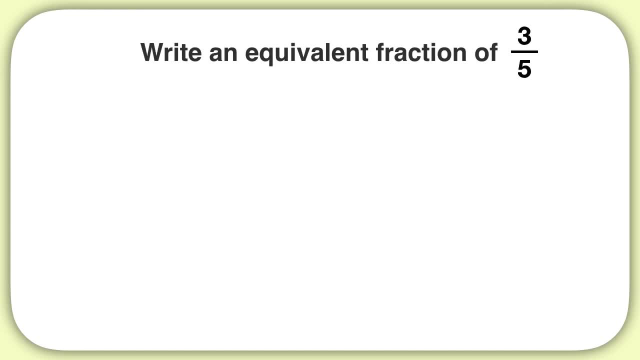 Here's another problem to practice with: Write an equivalent fraction of 3 fifths. Well, I could take my fraction 3 fifths, and which of these could I multiply it by? Well, Remember, I have to multiply the numerator and denominator by the same thing. so from: 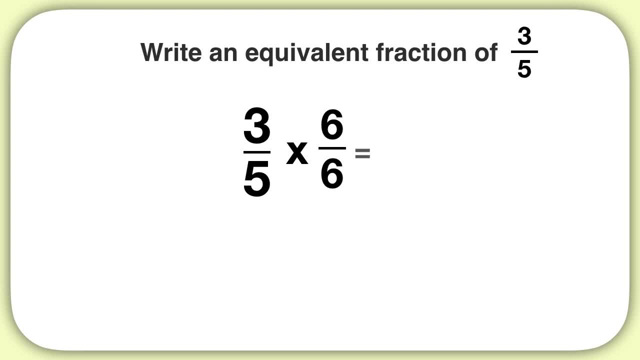 that list, the only option was 6 over 6.. What would this equal? Well, 3 times 6, that's 18, and 5 times 6, that's 30.. Three fifths is equivalent to 18 thirtieths. 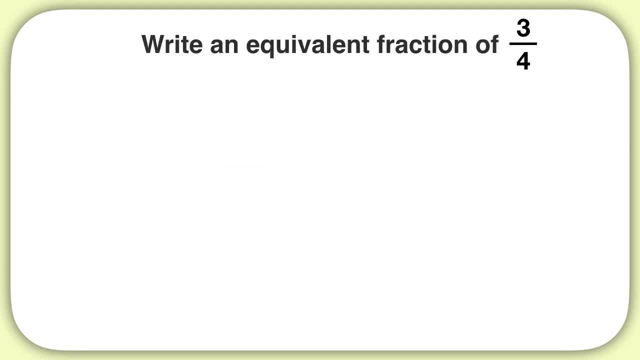 Now it's time for you to try on your own. Write an equivalent fraction of three fourths. You could have taken three fourths and multiplied by 2 over 2.. Three times 2 is 6, and 4 times 2 is 8.. 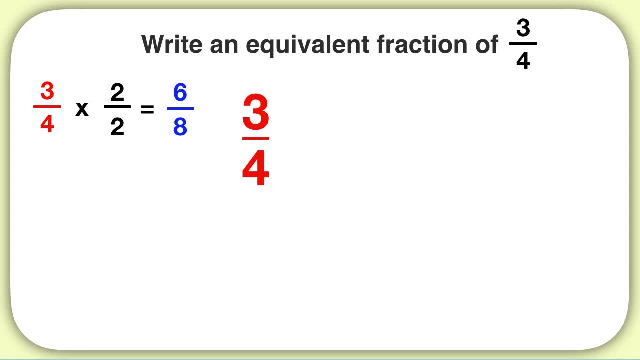 There's one equivalent fraction. Or you could have done three fourths and multiplied by 3 over 3.. Well, 3 times 3 is 9, and 4 times 3 is 12.. Nine twelfths is another equivalent fraction. 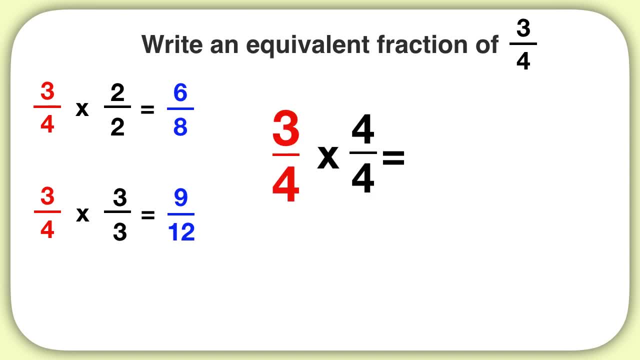 Or you could have taken three fourths and multiplied by 4 over 4.. Three times 4 is 12.. Four times 4 is 16.. There's another equivalent fraction. Here are three examples, but you could have picked other ones as well. 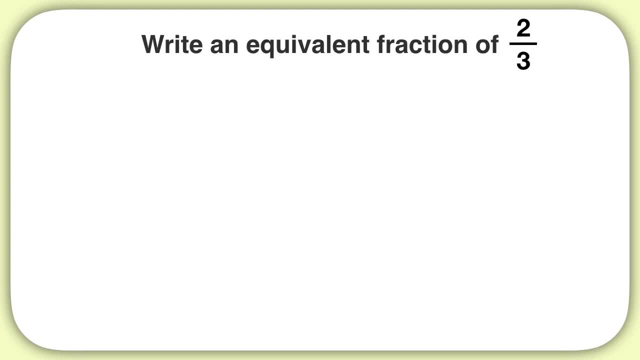 Now here's your last problem. for this video, Write an equivalent fraction of two thirds. You could have taken two thirds and multiplied by 2 over 2.. Two times 2 is 4, and 3 times 2 is 6.. 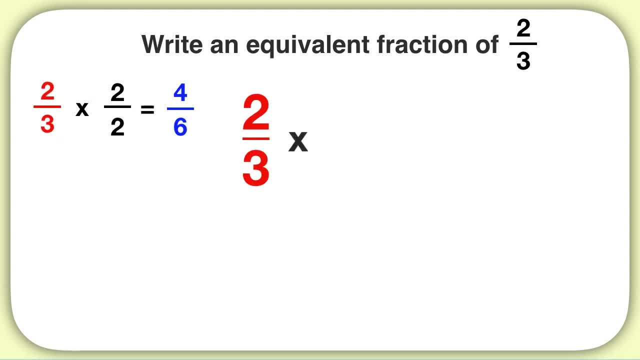 Four sixths is equivalent. Or you could have done two thirds times 3 over 3.. Two times 3 is 6, and 3 times 3 is 9.. Six ninths is another option. Lastly, you could have done two thirds times 4 over 4.. 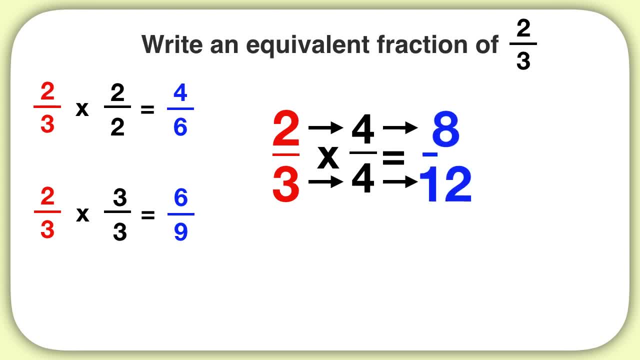 Well, 2 times 4 is 8.. 3 times 4 is 12.. Eight twelfths is another equivalent fraction. Again, you could have had other fractions if you multiplied by other numbers. Today, you learned how to find equivalent fractions by using multiplication.